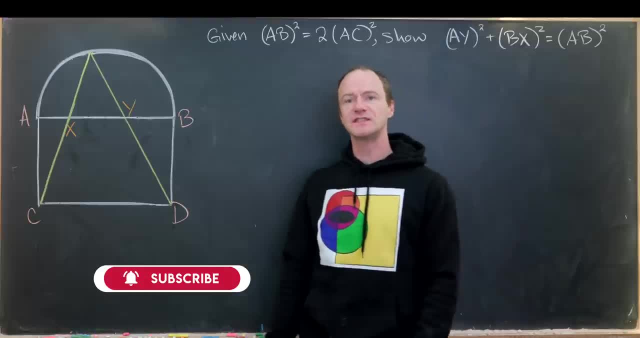 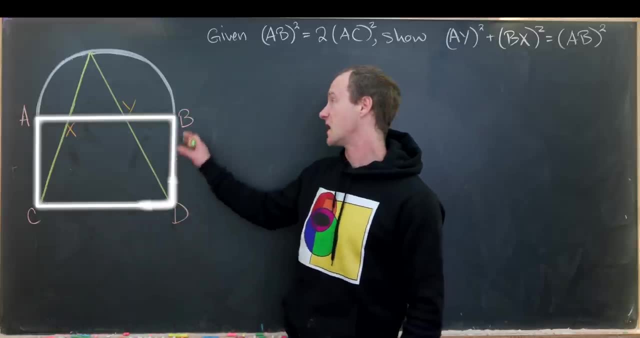 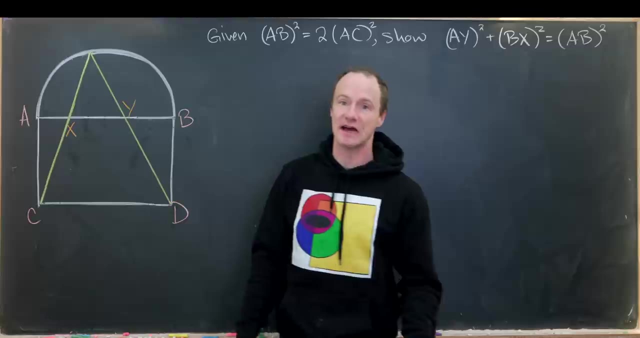 by putting the whole thing in a coordinate system. So let's see the setup that we have. We have a rectangle, ABCD, And kind of on top of that rectangle we have a semicircle, so that's a half circle, So that AB is a diameter of that semicircle. 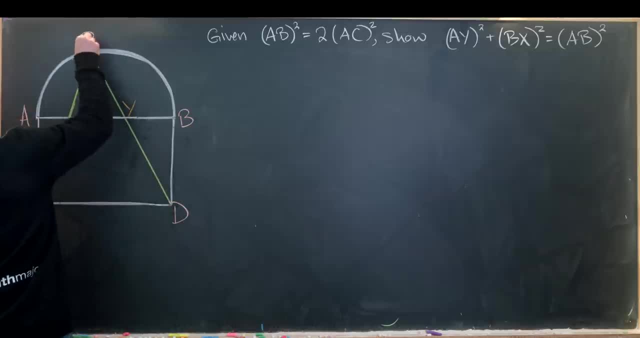 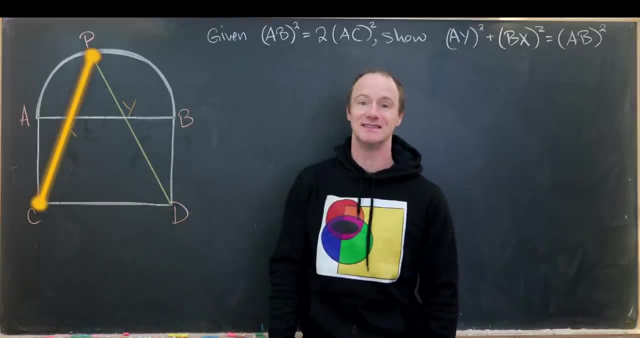 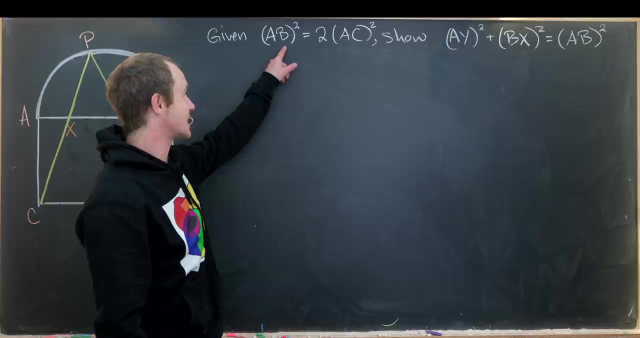 Next, we put a point up here, P on the semicircle, And we connect line segments to this vertex C and this vertex D. So that's our setup at the moment. And then what we have is that, given the line segment length AB, squared is twice line segment length AC. 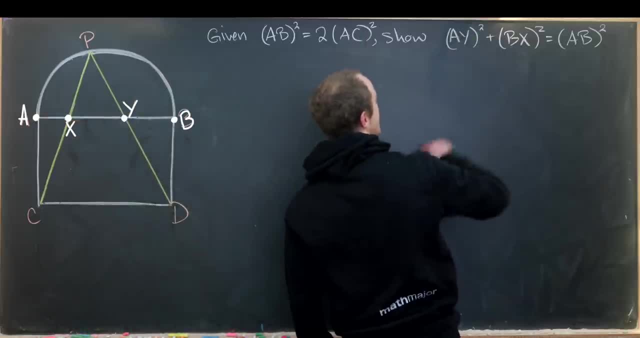 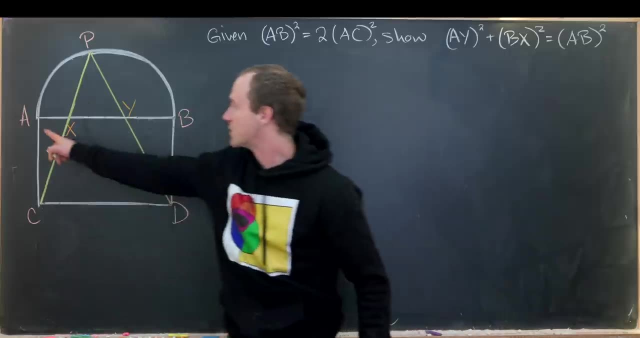 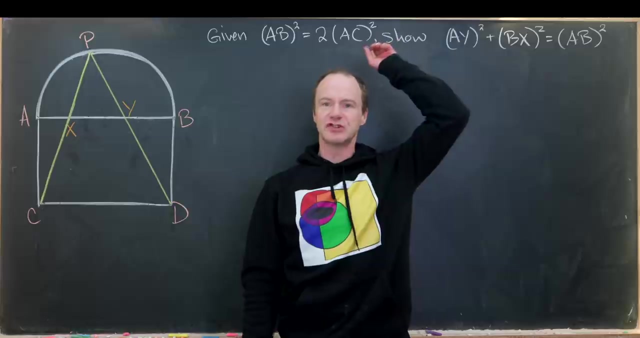 squared. we want to show that AY squared plus BX squared equals AB squared. So let's look at those measurements. So this length right here, A to B is square root of 2, this length right here, A to C, But I've just written it up there like in terms of squares, so we don't have square root. 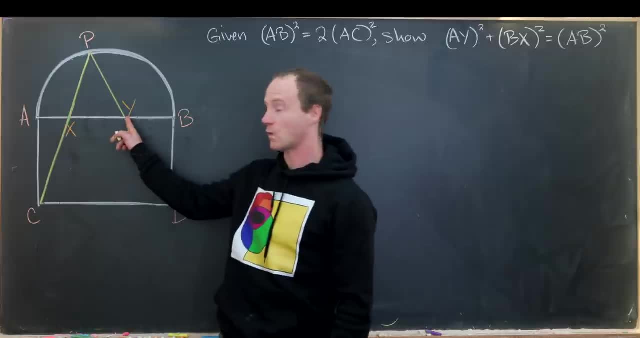 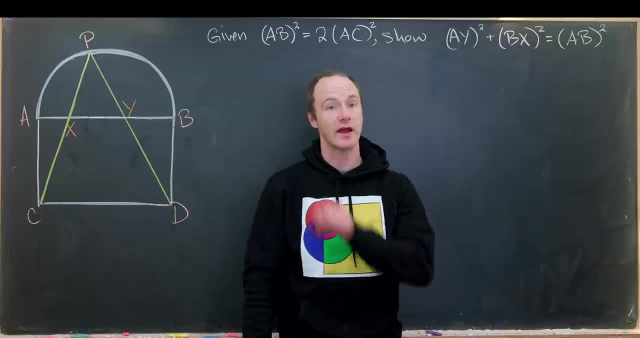 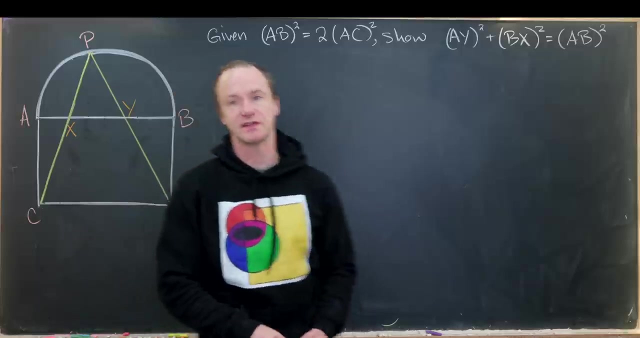 roots. Then we want to show that this length right here, A to Y squared plus B to X squared, is equal to A to B squared. So that's like our final goal. Okay, so, like I said, we're going to put this whole thing in a coordinate system. 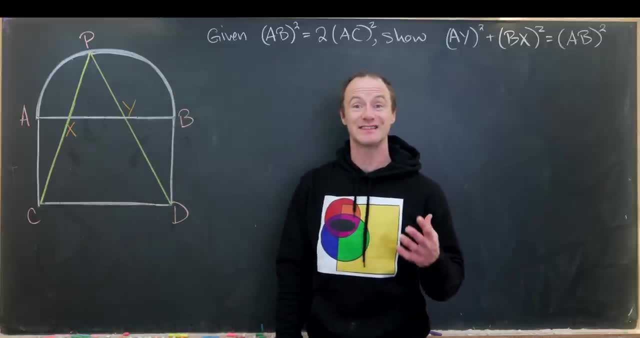 and I tried this a couple of different ways, and I think the simplest place to put the origin is at the midpoint of A and B. So let's do that. So let's see the midpoint of A, B and B. So that's our final goal. So let's do that. So let's see the midpoint of A and B. The first thing we do is: how do we know that this will be an accordion? This is where we put it at the midpoint of A and B, And when we try to put it to the square root, we don't know if we'll be able to see the whole thing at the same time. 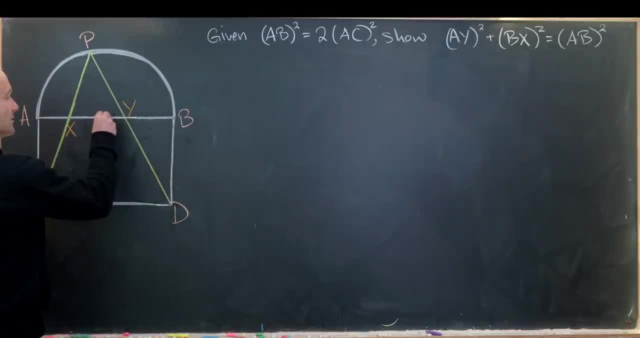 So let's do that. So let's see, the midpoint of A and B is right about here, So I'll put my origin right there. So that means B and A both lie along the x-axis. Furthermore, let's scale this so that: 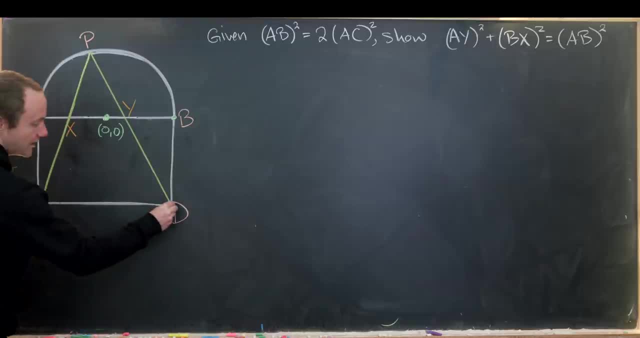 the length of AC is 1.. So that's going to help us. So if the length of AC is 1, that means the length of AB is the square root of 2, which means B has coordinate square root of 2 over 2 comma 0.. 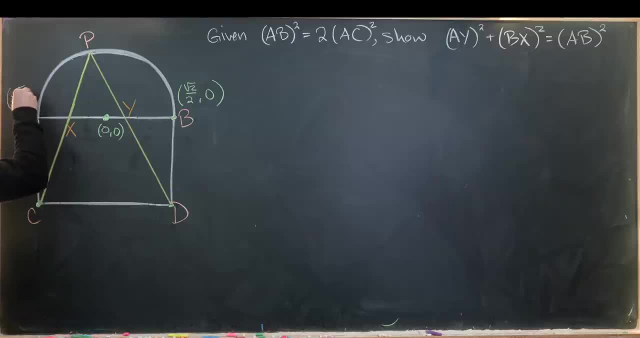 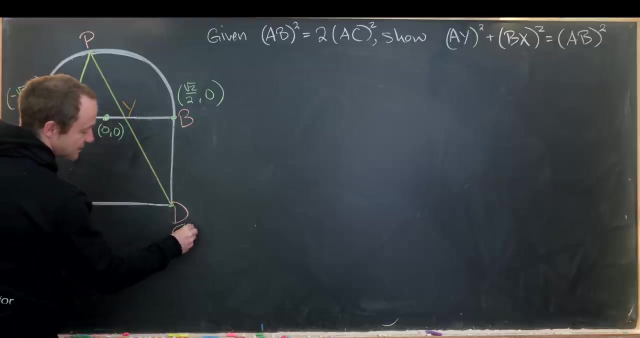 And then A has coordinate negative square root of 2 over 2 comma 0.. Now we can fill in the rest pretty easily. So let's see: C has coordinate negative square root of 2 over 2 comma negative 1.. And then this has coordinate square root of 2 over 2 comma 1, because that's below the 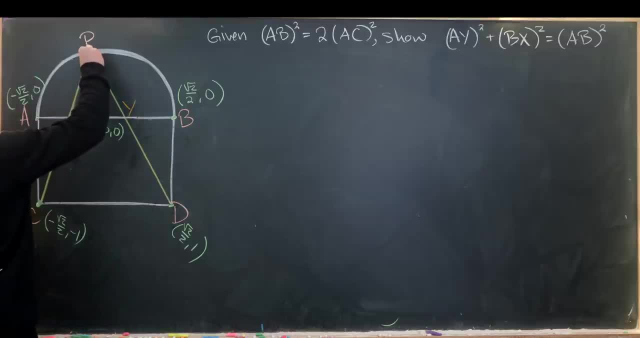 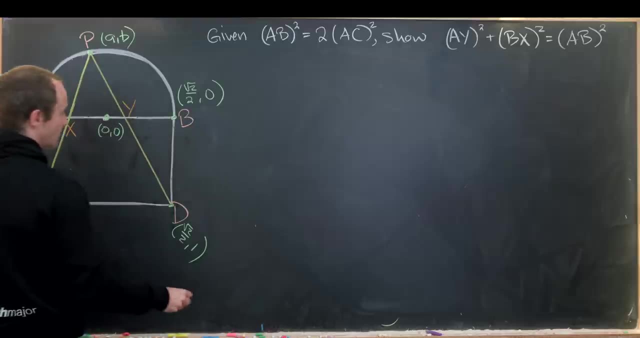 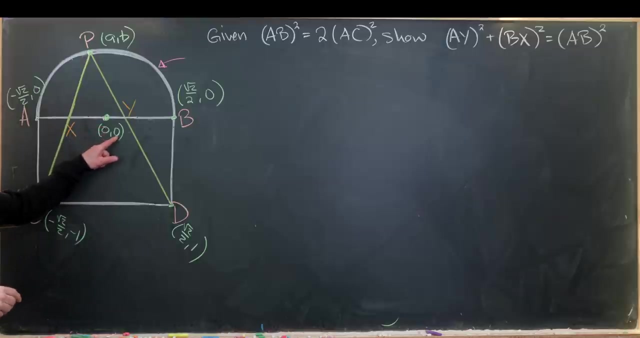 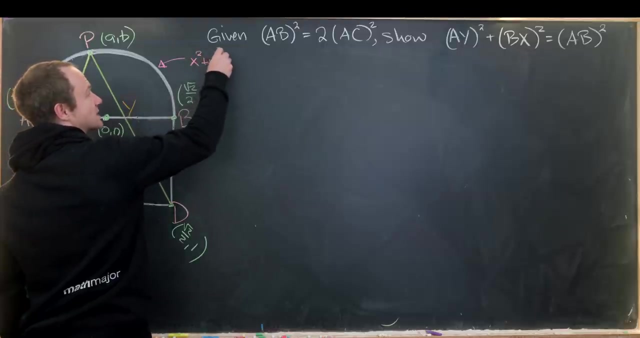 x-axis And then P up here has a fairly general coordinate. I'll call this AB, but it's on that circle. Furthermore, we can easily write an equation of this circle, given that it has center 0,, 0, and it has radius square root of 2 over 2.. So that means it has equation x squared plus. 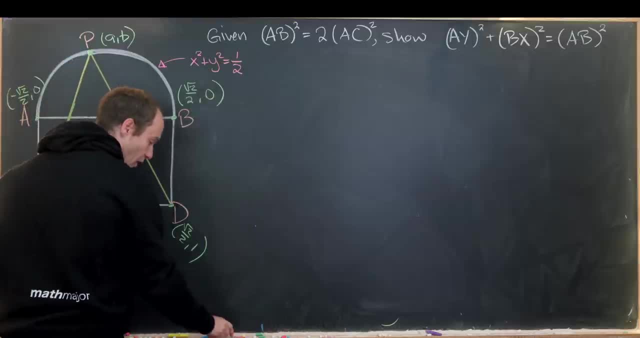 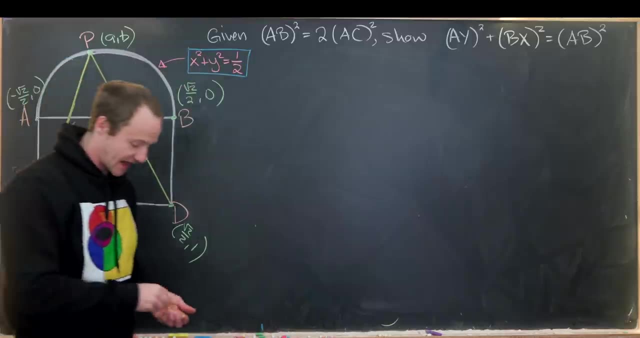 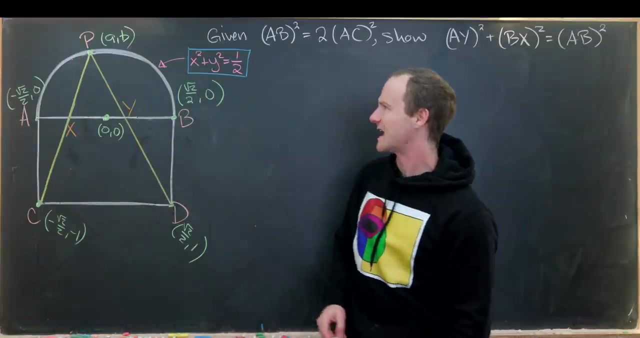 y squared equals 1 half. 1 half is the square of the square root of 2 over 2.. So that means these numbers, A and B, satisfy that equation. We'll use that a bit later. So A squared plus B squared is equal to half. So now let's dive into these lines that we have. We want to first: 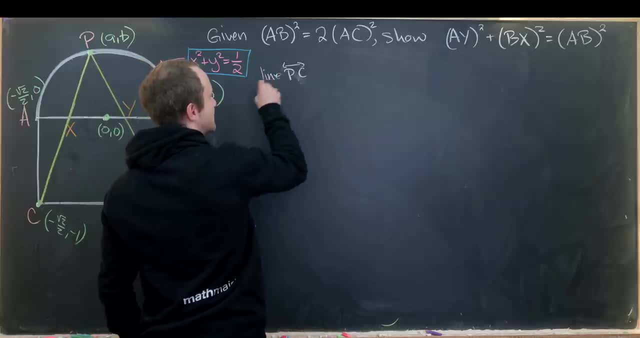 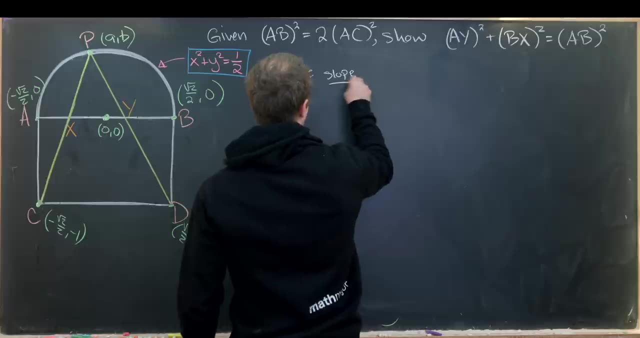 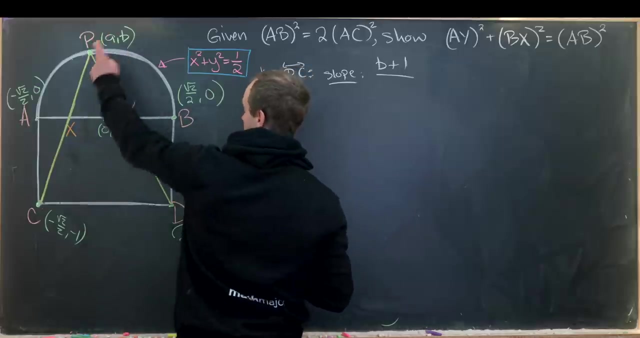 look at line PC. Okay, So let's first calculate its slope. So the slope of line PC, So that will be the difference in the y-coordinates. So that gives us B plus 1 over the difference in the x-coordinates. So that'll be A plus the square root of 2 over 2.. 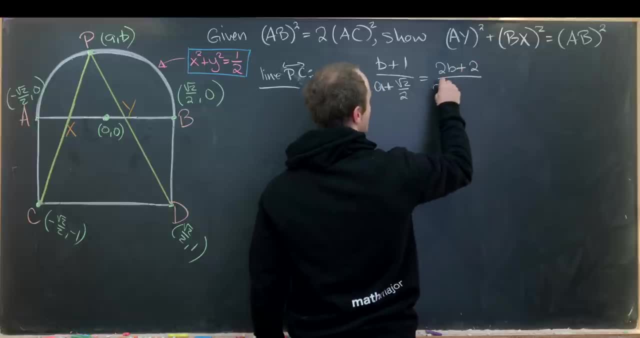 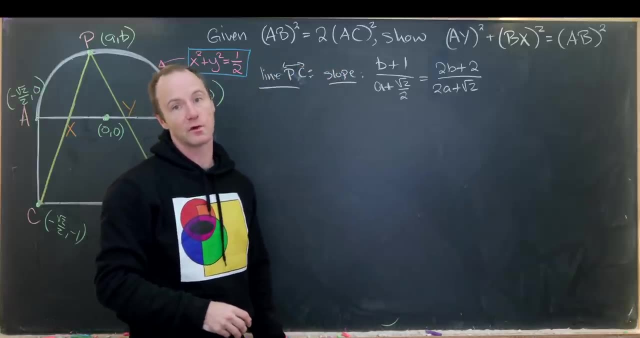 We can simplify that to 2B plus 2 over 2A, plus the square root of 2, if we'd like to. Okay, Then we can use the point-slope form of a line to write down an equation for this line. 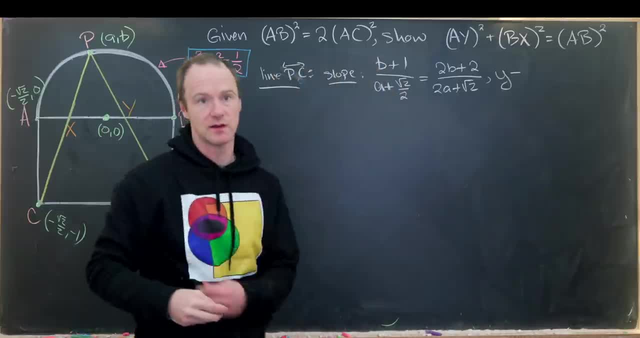 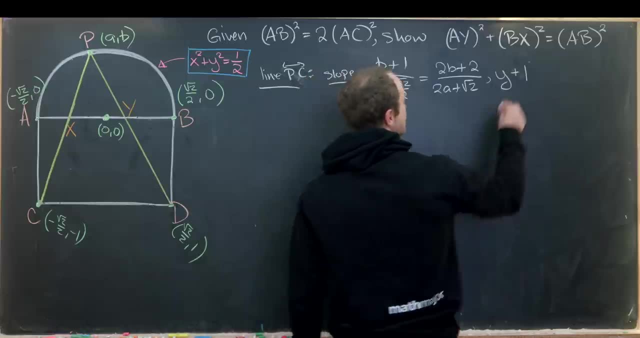 So we'll have y minus a y coordinate. maybe we'll use this y coordinate right here, so that'll be y plus 1, because the y coordinate is negative. 1 equals slope, so that's 2b plus 2 over 2a plus root 2. 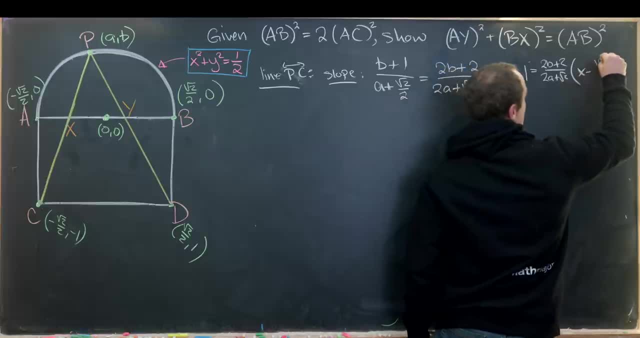 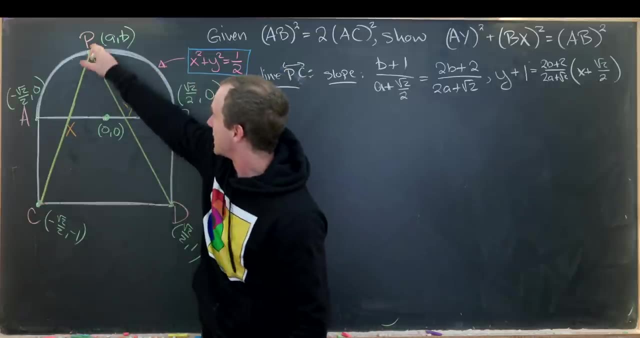 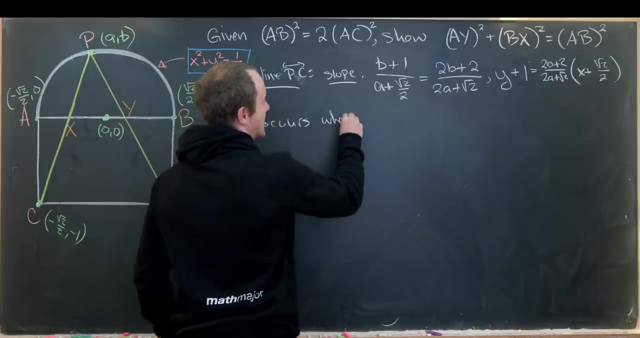 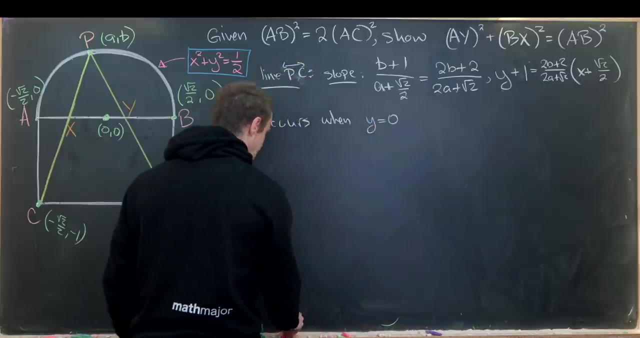 and then x minus the x coordinate, which is the square root of 2 over 2, but it's negative, thus changing that to a plus. now notice that this line intersects at x, and so the point x occurs when our little x equals zero, or i should say our little y equals zero, because we're along the x. 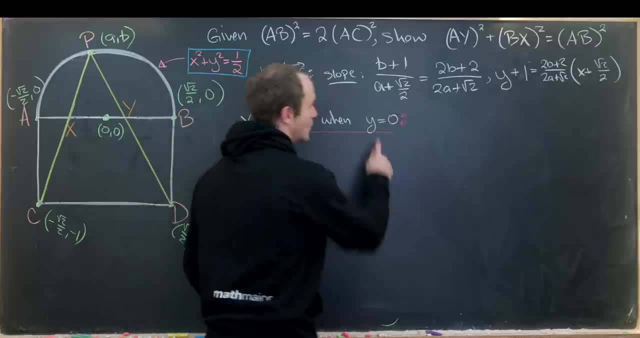 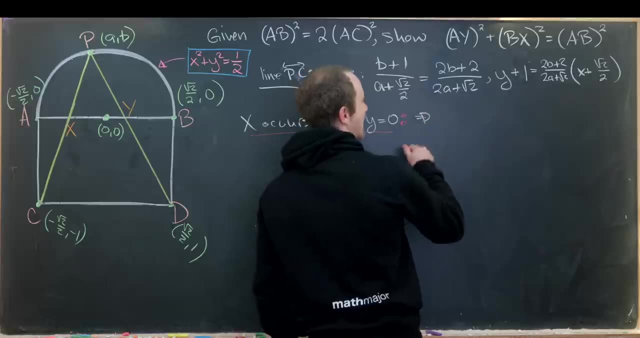 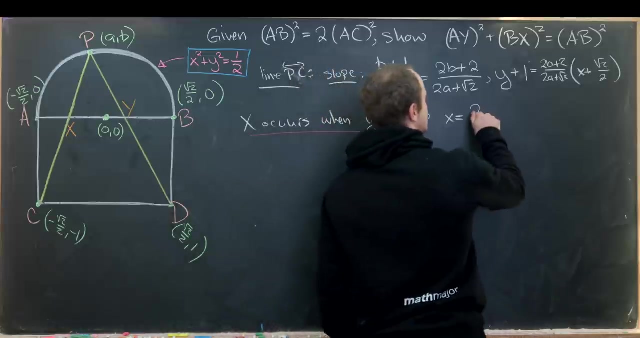 axis. so that's important. so we plug y equals zero into this equation and we can solve for x. so let's see, solving that first for x, we get little x equals. so let's see, we'll end up with 2a plus root 2 over 2b plus 2. 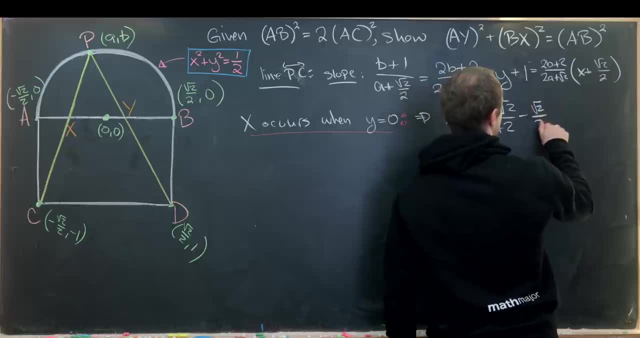 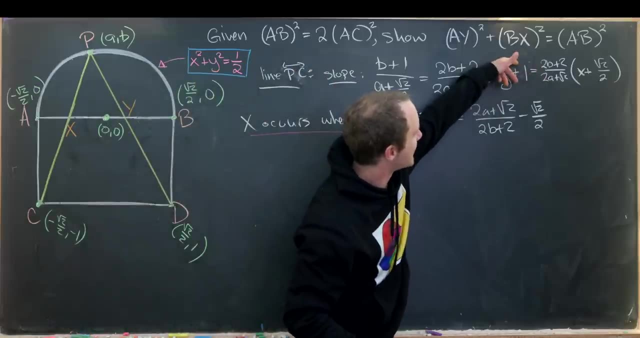 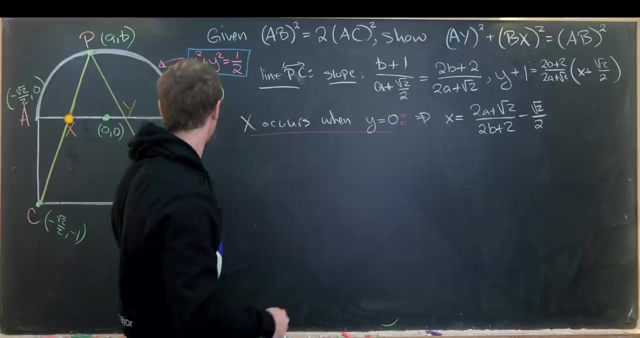 and then minus the square root of 2 over 2. okay, so just to reiterate, that's setting y equal to zero, then we would multiply by the reciprocal of this and subtract that root 2 over 2 over. but really what we want is the distance from b. to x, so that's 2b plus 2 over 2 and then minus the square root of 2 over 2, so that's 2b plus 2 over 2, and then minus the square root of 2 over 2 and then minus the square root of 2 over 2. 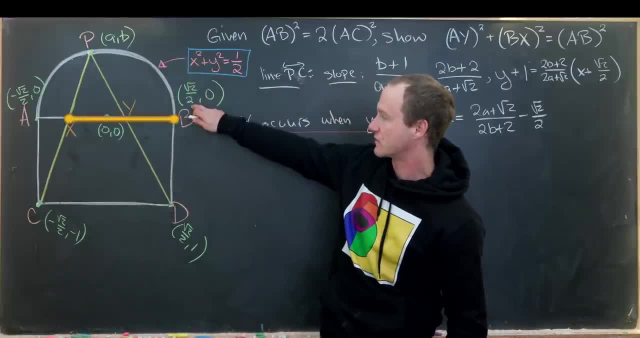 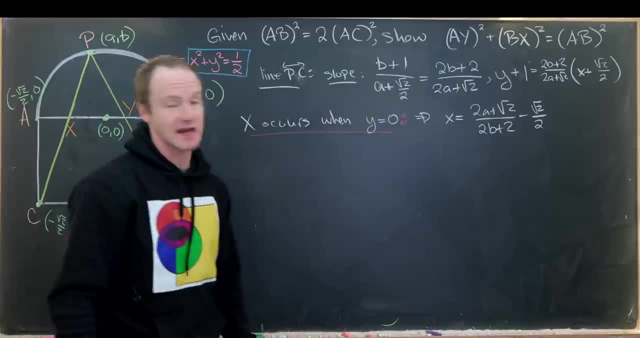 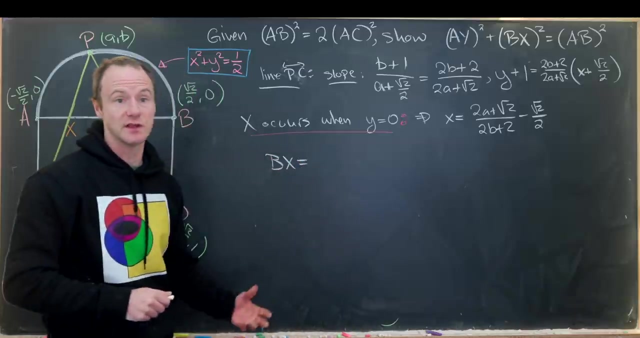 x, keeping in mind that b has this equation right here. so we need to do this x coordinate here: root 2 over 2, minus this x coordinate here, given that they're all along the same horizontal line. so that tells us that bx, or the length bx, is equal to the square root of 2. 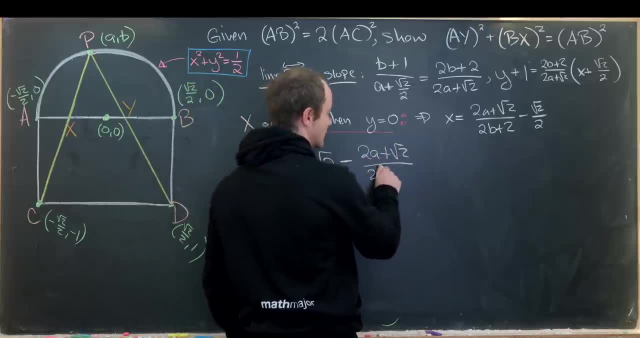 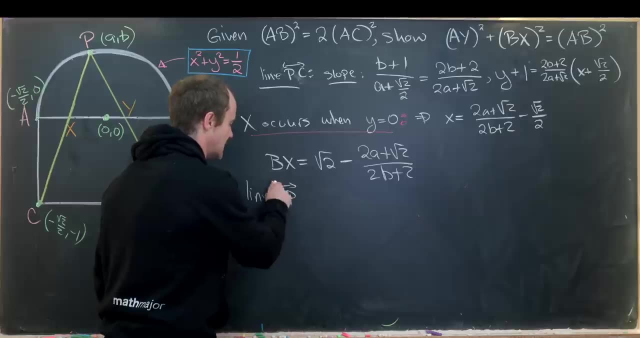 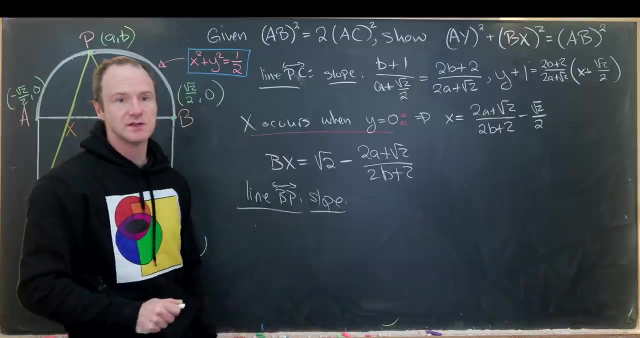 minus 2 plus a root, 2 over 2b plus 2. and now let's dive into the next line, so that'll be line bp. so we need to calculate the slope and the equation of that as well. so let's see: the slope in this case would be the difference in the y coordinates. so this should be: 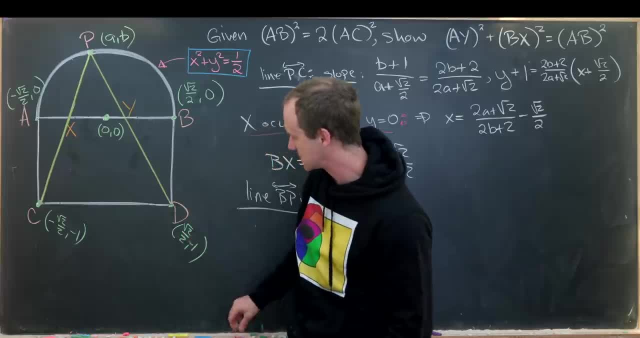 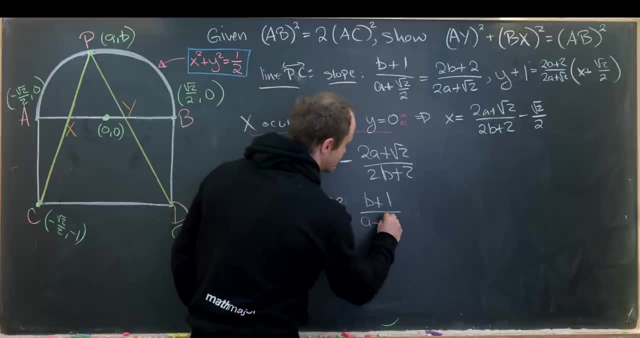 a minus 1 down here. i think i said that but i forgot to write it. so i have b plus 1 again, but now it's going to be over a minus root, 2 over 2. we might simplify that to 2b plus 2 over 2. 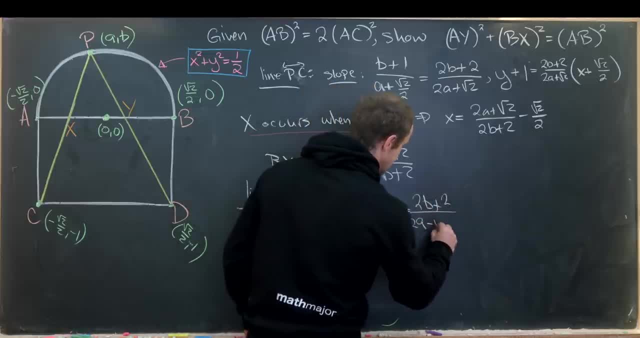 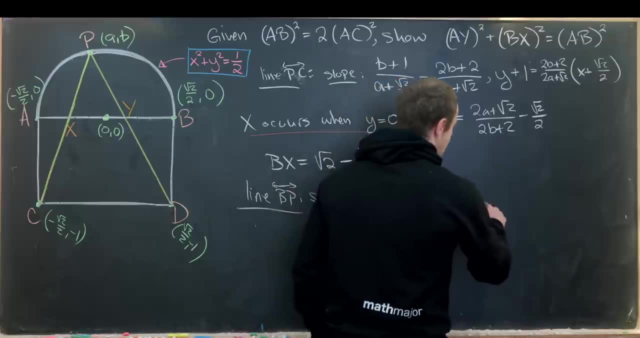 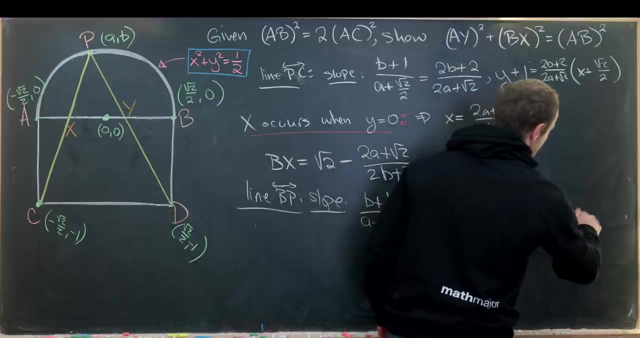 a minus the square root of 2, just to make it look like the other one. now we can use point slope form again and we'll get y plus 1 equals this slope, 2b plus 2 over 2a minus root 2, and then we'll have x. 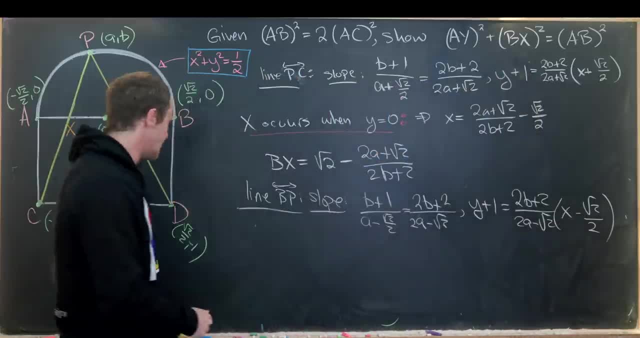 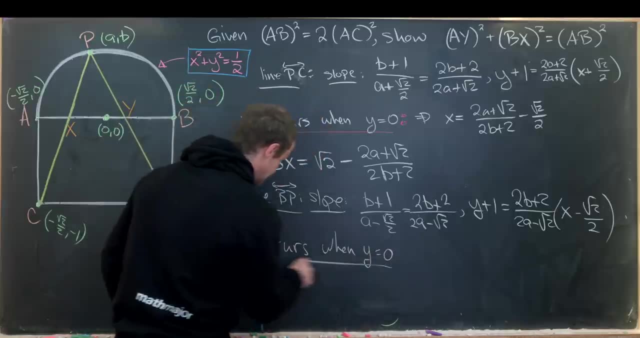 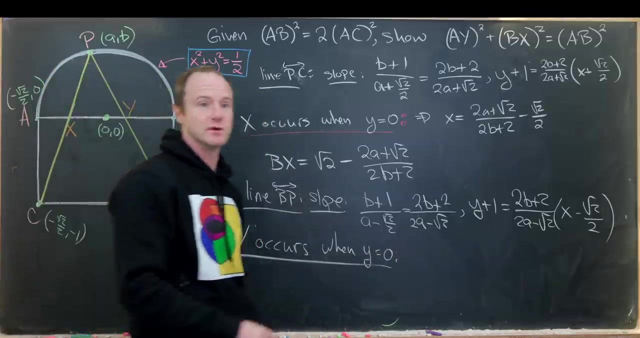 minus square root of 2 over 2. now we want to find out the coordinate y. so y occurs when little y is equal to zero, kind of in parallel to what's going on up here. so solving for x, we'll get. x is equal to, in this case it is. 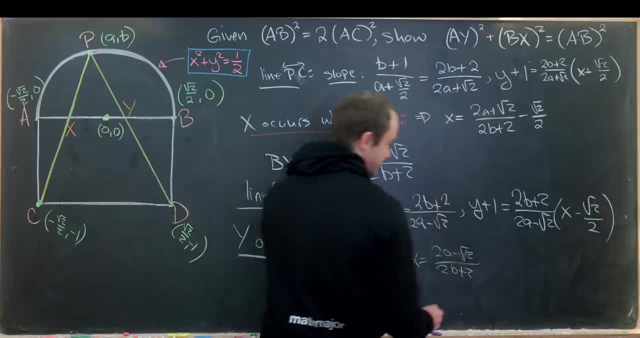 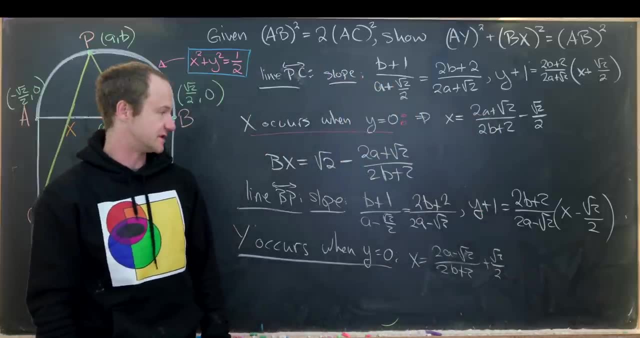 2a minus root, 2 over 2b plus 2, and then we'll have plus the square root of 2 over 2. so we get that just from setting y equals zero into this equation, and now we can calculate ay. so that's. 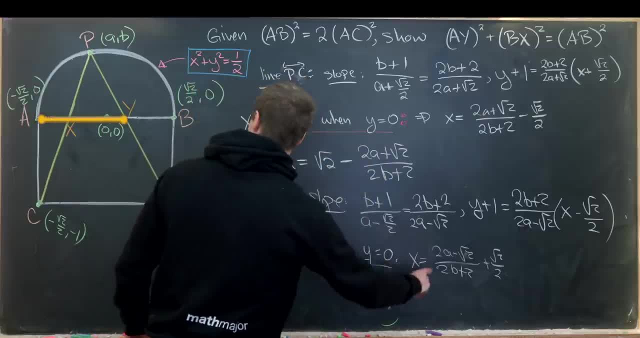 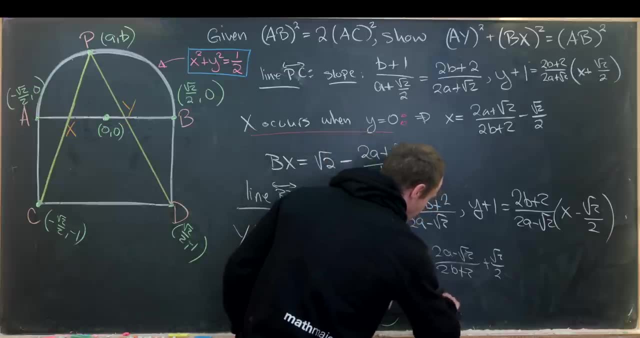 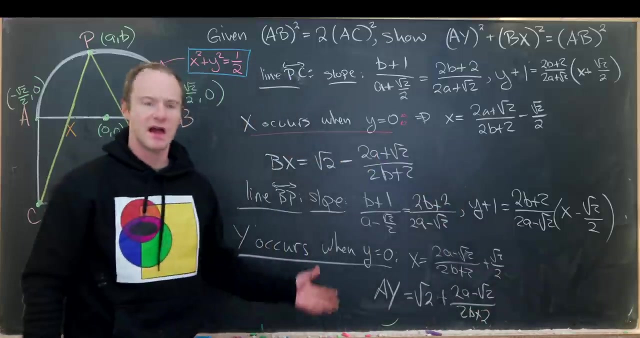 going to be the distance between this coordinate along the x-axis, and then we'll have x equals 2 over 2, and then we'll have y equals 0 over 2, and then we'll have plus the square root of 2 plus 2a, minus root 2 over 2b plus 2, again doing the difference in the x. 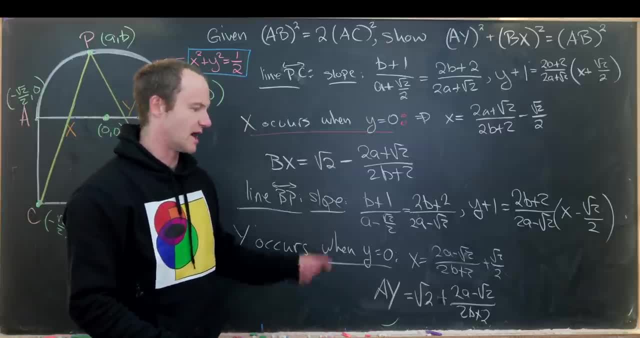 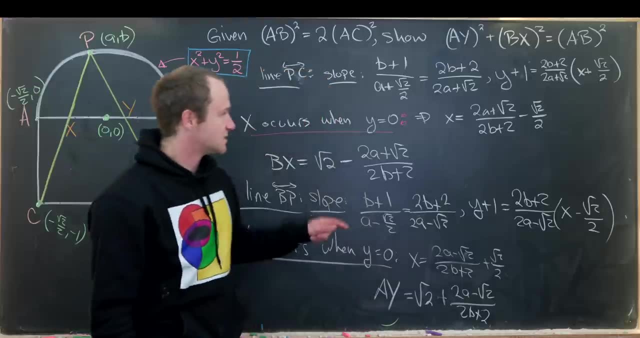 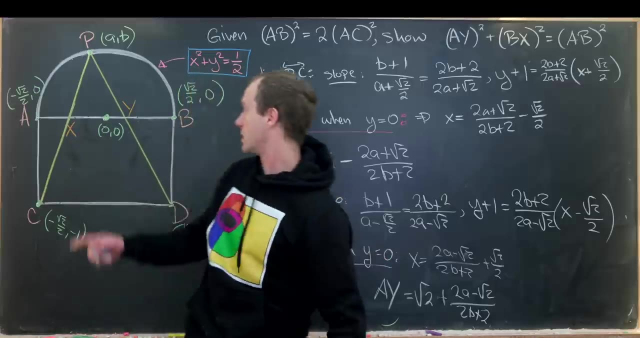 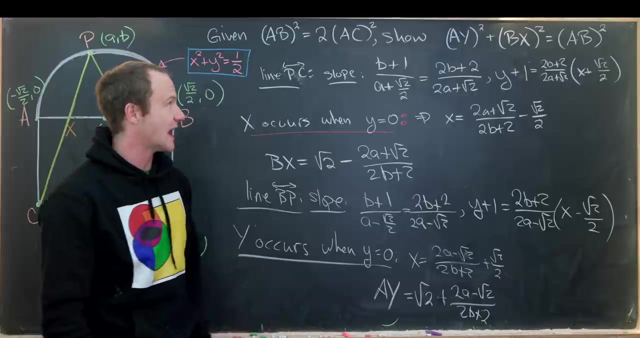 coordinates, just as we did in this one up here, keeping in mind that the y coordinates of capital x and capital y are both zero. so these are the x coordinates of capital x, right here, and then, like i said, this was the x coordinate of capital y. okay, so now we've got a form for a- y and b- x. 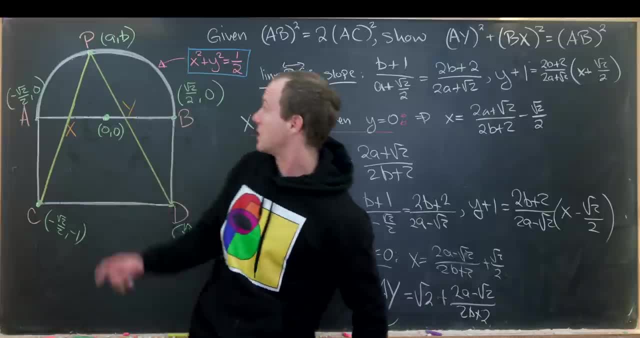 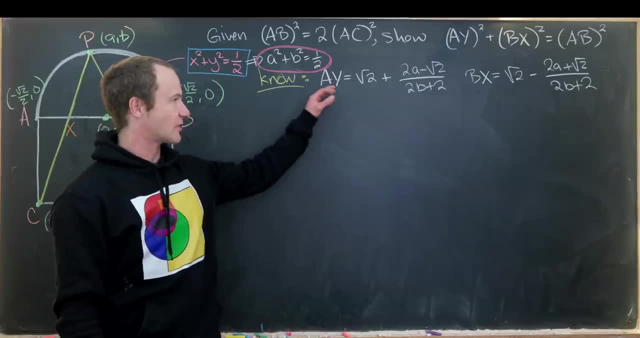 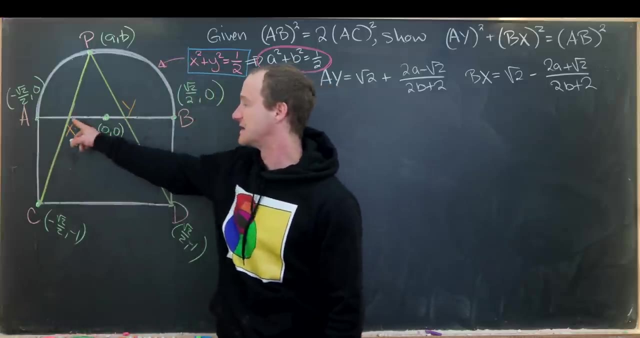 and we know that a and b are on this circle, so they satisfy this equation. so all that's left is to do a quick calculation. so on the last board we calculated values for a, y and b, x, that's the distance of this line segment from a to y and b to x. we did that by getting close to the x-axis. 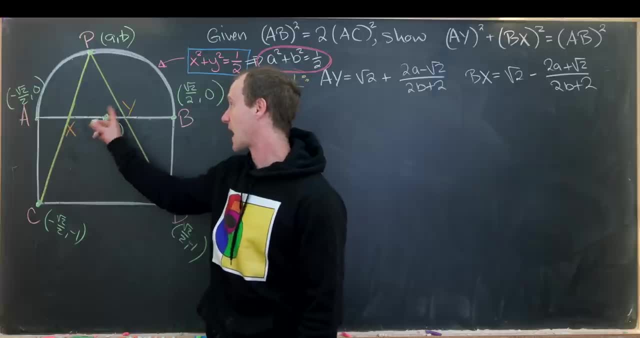 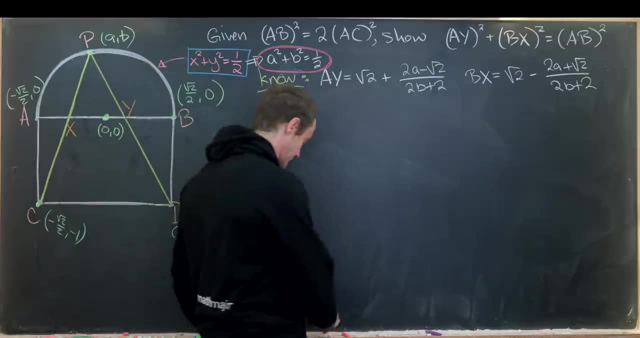 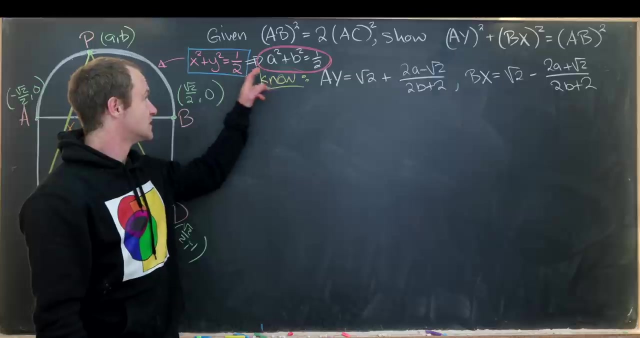 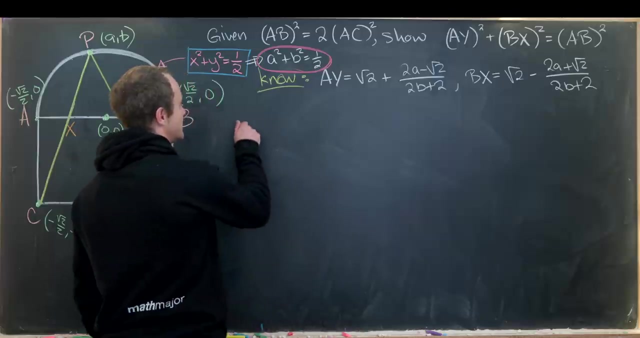 so now we're ready to finish this thing off and, like i said before, we'll use the fact that the coordinate a comma b is on our circle, so that means it satisfies this equation: a squared plus b squared equals half. okay, so now let's get to it. so we have a y squared plus b x squared. 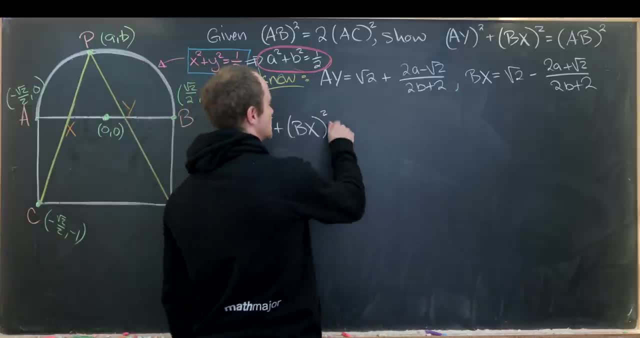 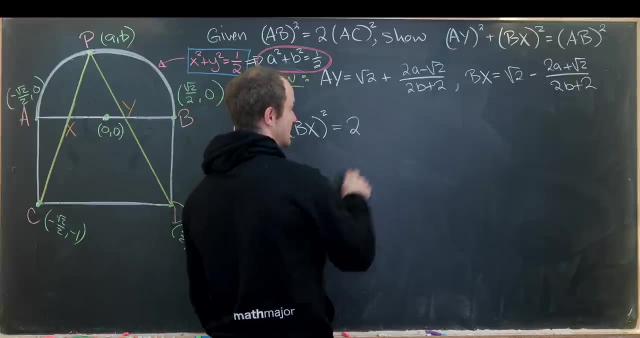 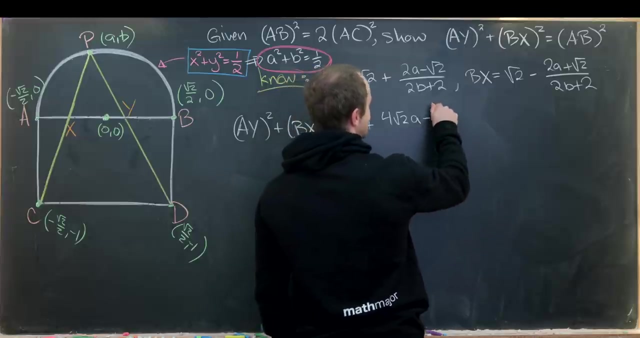 that's, like i said, our final goal. so let's multiply these things out and see what we get. so a y squared will be 2- that's from squaring the square root of 2- and then we'll have plus 4 times the square root of 2, times a minus 4: that's what we get from doing 2 this term. 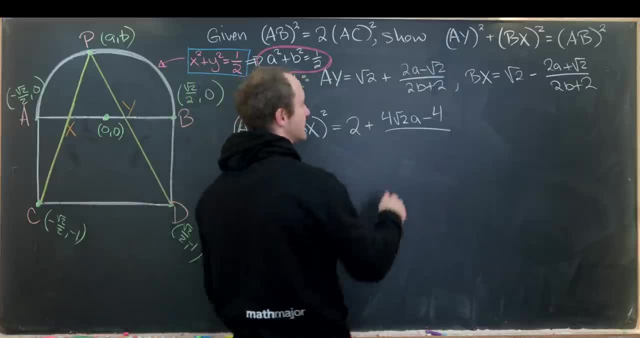 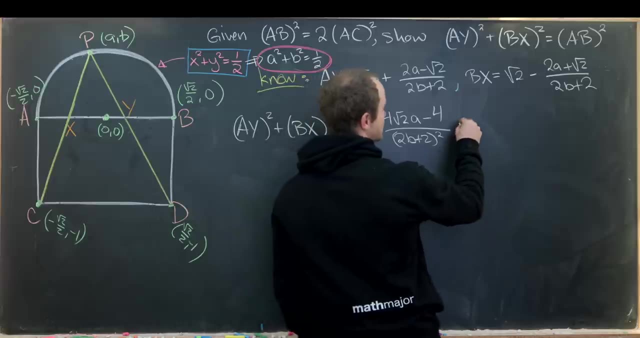 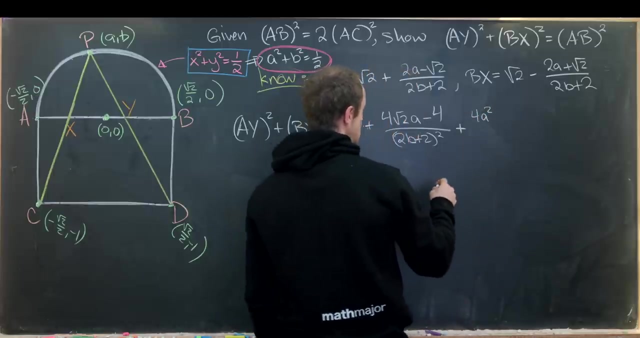 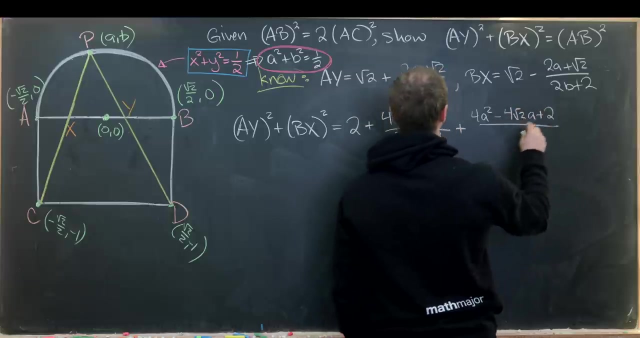 times this term, just by binomial squared formula, and then we have a 2b plus 2 in the denominator. then we have to square this term. so that's going to give us something like this: so we'll have 4a squared and then minus 4 times the square root of 2 times a plus 2, and this is all over. 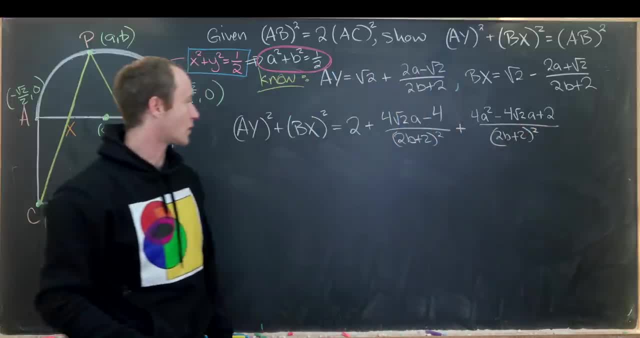 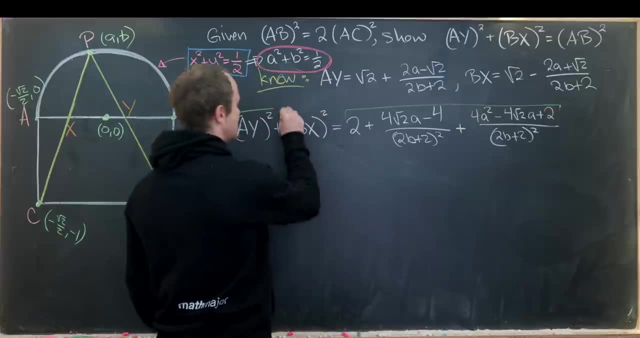 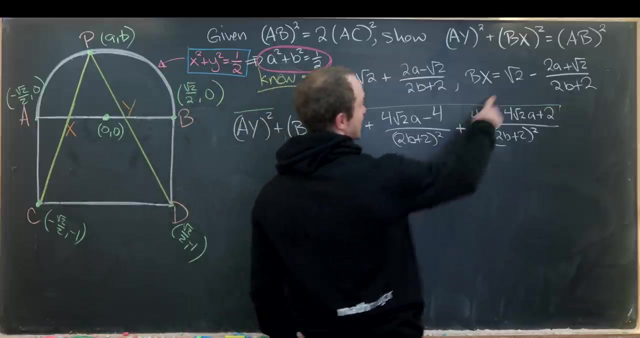 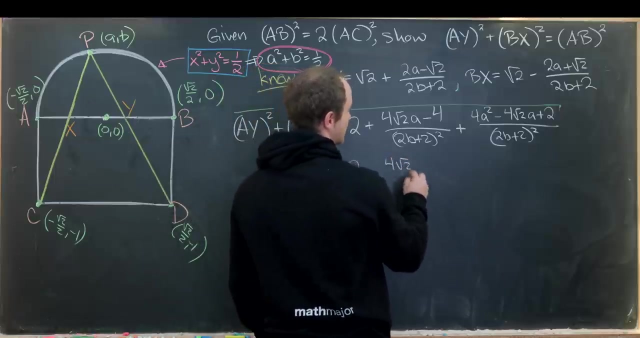 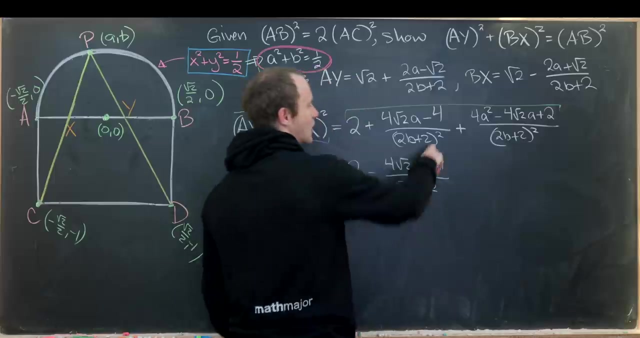 2b plus 2 squared just as before. okay, so that so far is our a y term. so now let's multiply out our x term and see what we get for that. okay, so we'll start with a 2 again from this being squared, and now we'll subtract 4 times the square root of 2 times a plus 4 over 2b plus 2. oh, this shouldn't. 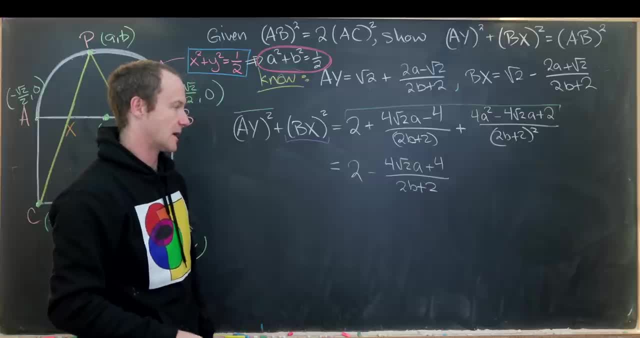 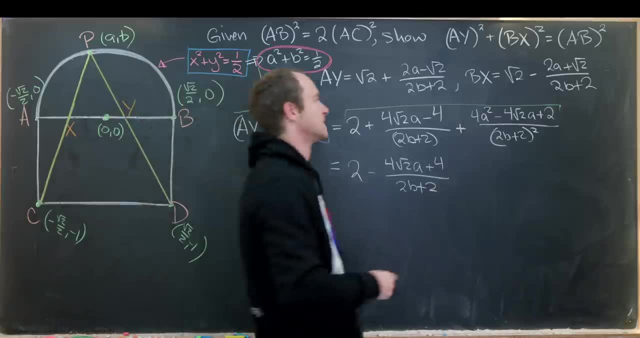 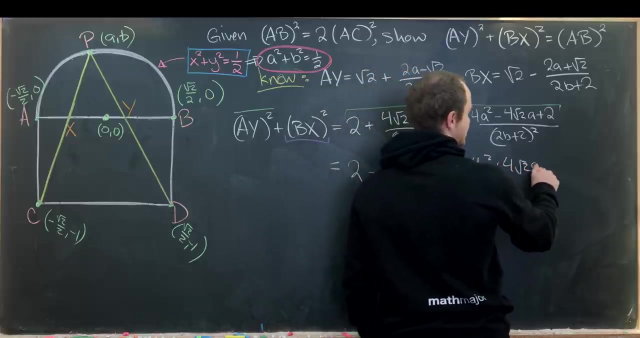 have been squared. that was my mistake from the last one. okay, so that's subtracting twice the cross term here, just from multiplying out binomial, and then for this last bit, we'll have plus 4a squared, plus 4 square root of 2a plus 2 all over. 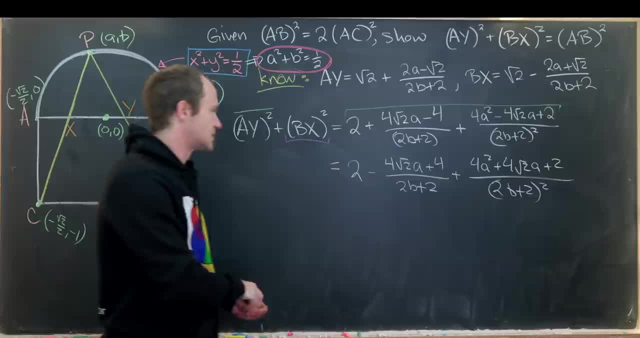 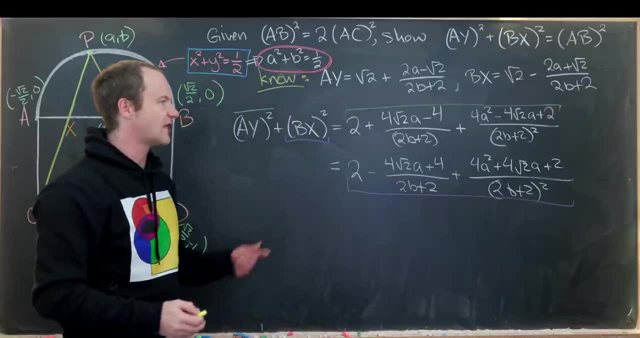 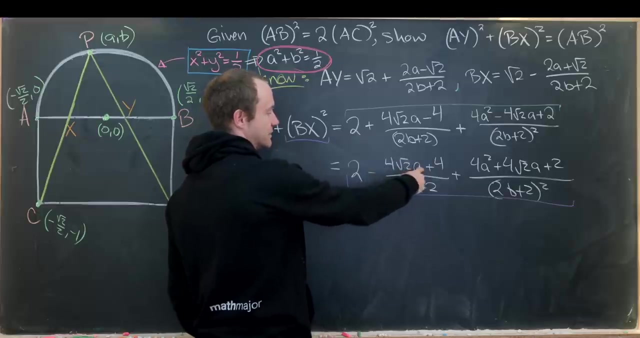 2b plus 2 squared. so just to reiterate, that is what we get for our bx squared. and now let's simplify and cancel as much as we can. so here we have a 4 root 2a. here's a negative 4 root 2a. 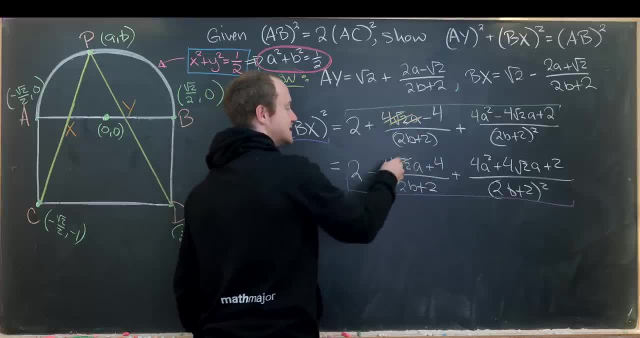 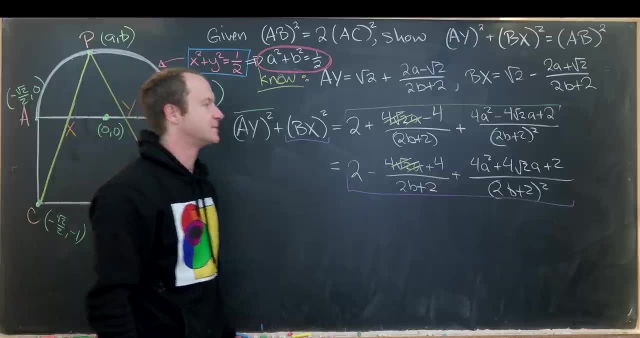 they're both over the same denominator. so we're going to subtract 4 times the square root of 2, so that means these two will cancel each other, which is good. having these squares square roots of 2 in here is not super nice. then the same thing here. here we have a negative 4 root. 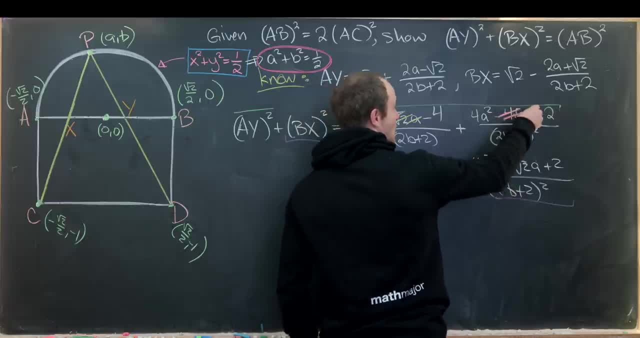 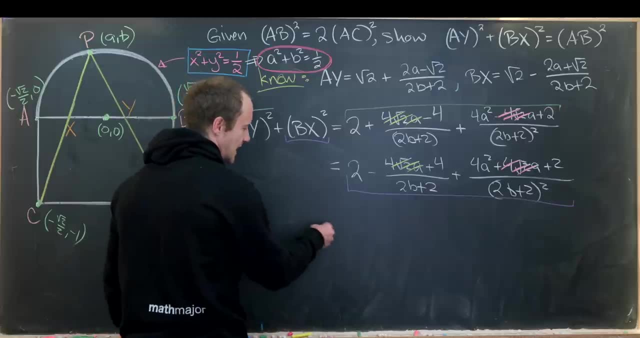 2a, a plus 4, root 2a, and they're again over the same denominator, so those will cancel as well. okay, so now let's combine everything that we can, so 2 plus 2 will give us 4, and then let's see we'll. 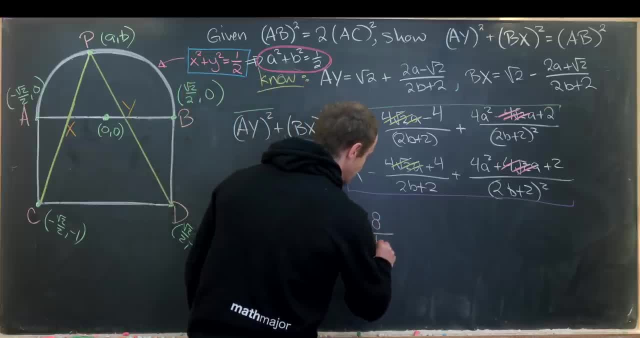 have negative 8, and then we'll have negative 8, and then we'll have negative 8, and then we'll have negative 8 over 2b plus 2, so that'll become from this negative 4 and this negative 4, and then next. 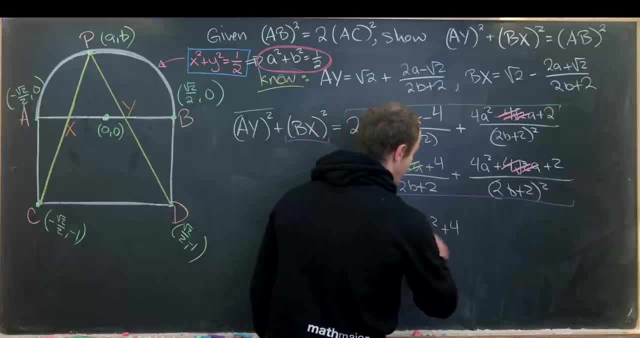 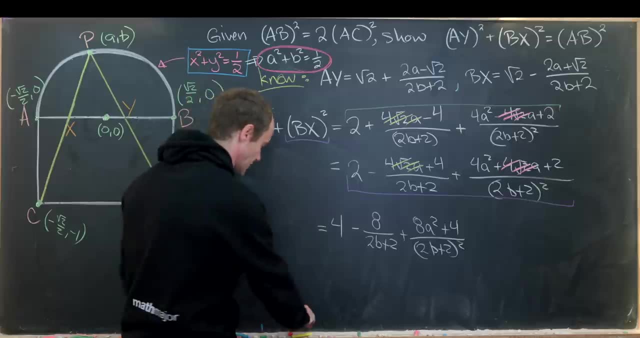 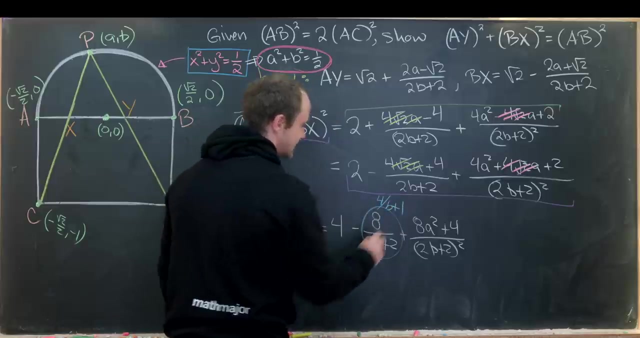 we'll have plus 8a squared plus 4 over 2b plus 2 squared. but i can do some pretty quick simplification here, so this term can quickly simplify to 4 over b plus 1 just by factoring a, 2 out of the numerator and the denominator and then 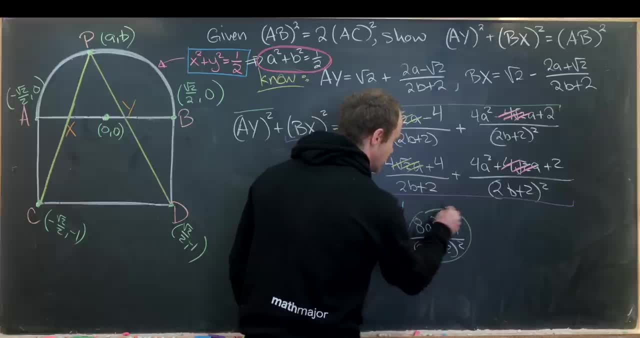 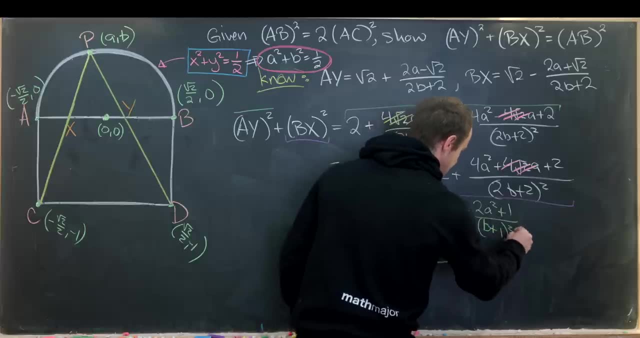 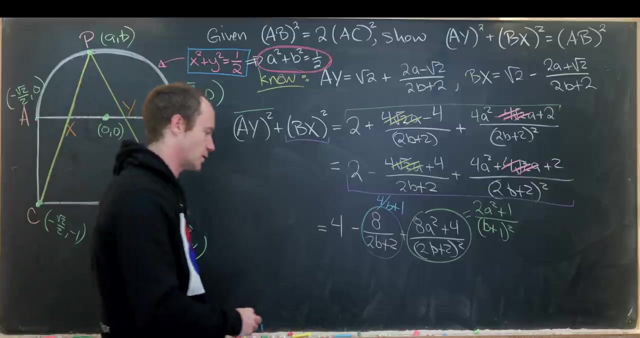 furthermore, by factoring a 4 out of the numerator and the denominator, here i'm left with 2a squared plus 1 over b plus 1 quantity squared. now i'm in a place where i can put everything into a common denominator of b plus 1 squared, so that's going to give me 4 times b plus 1. 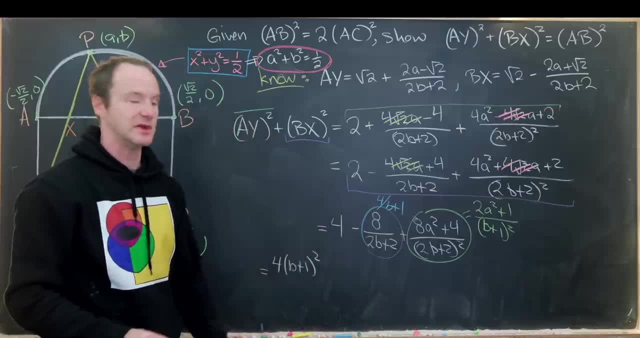 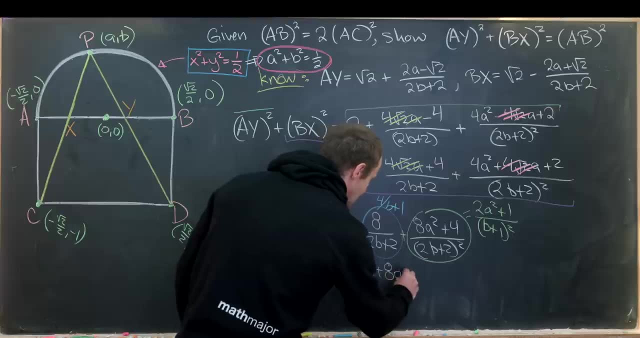 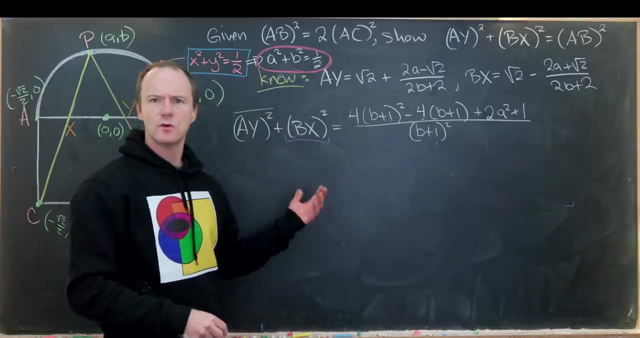 squared again, putting this one with a denominator of b plus 1 minus 8 times b plus 1, and then finally plus 8a squared plus 4. this is all occurring over b plus 1 squared like that. so quickly fixing a typo that was on the last board leaves us with the following object in the: 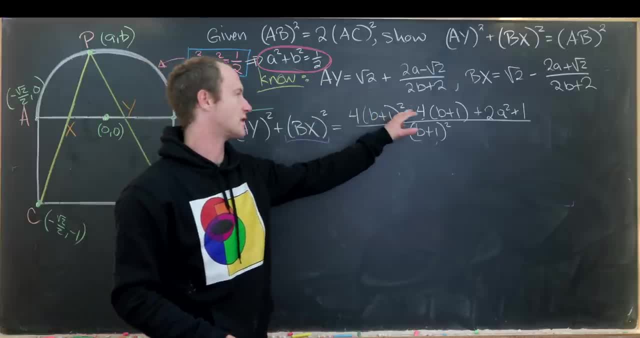 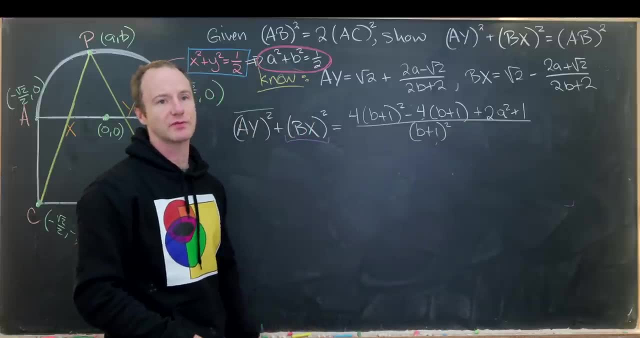 numerator. we have 4 times b plus 1, squared, minus 4 times b plus 1, plus 2 times a squared plus 1, all over b plus 1 squared. now we're ready to start simplifying. we'll make use of this, like i pointed.